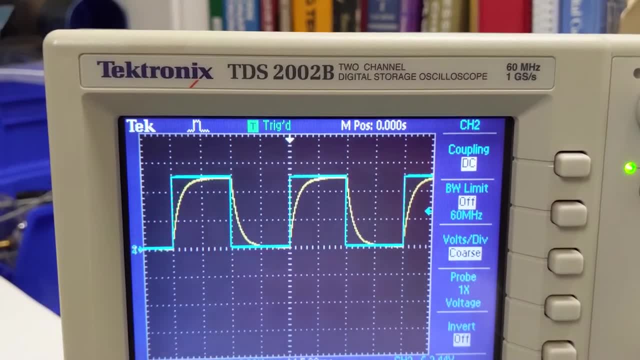 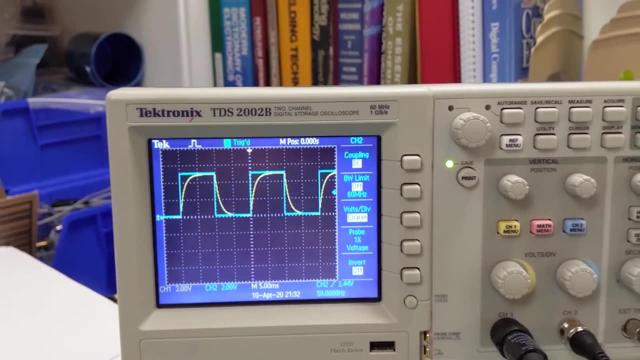 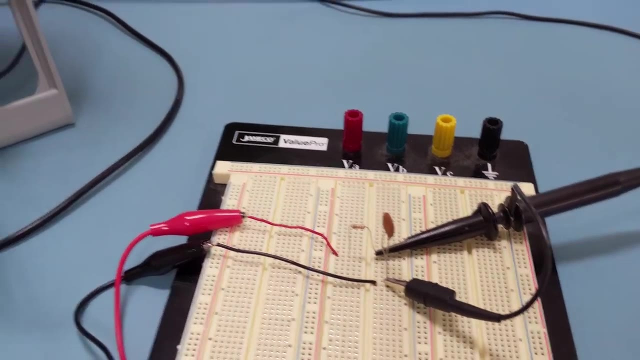 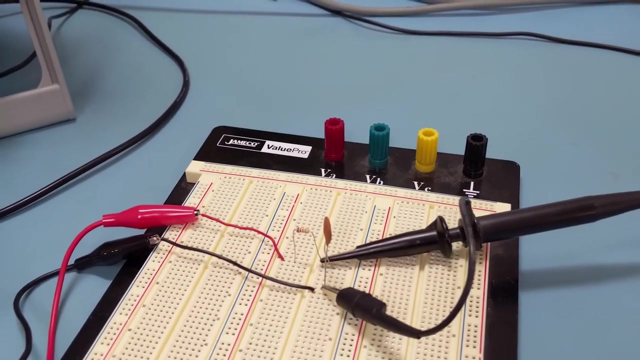 the signal goes into the capacitor, it charges, And then, when it drops down to zero, it discharges. It's kind of cool to see those two overlapping, and pretty cool to be able to see what the circuit's doing. And so let's do some math to figure out what the capacitance is of this capacitor. 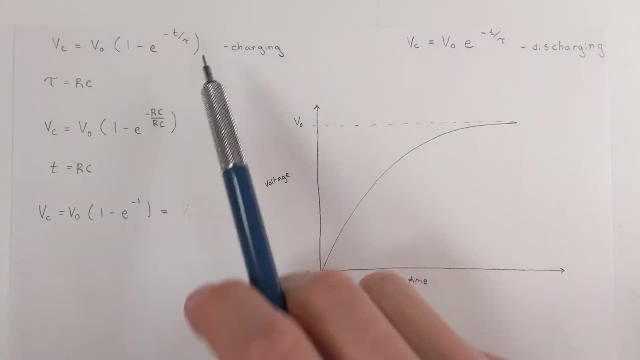 Okay, so we're going to be using this equation for this problem. You can also use this equation if the capacitor is discharging, but since we're working with a part of the wave that is increasing or charging, We're going to be using this equation, And so what we're going to do, let me walk you. 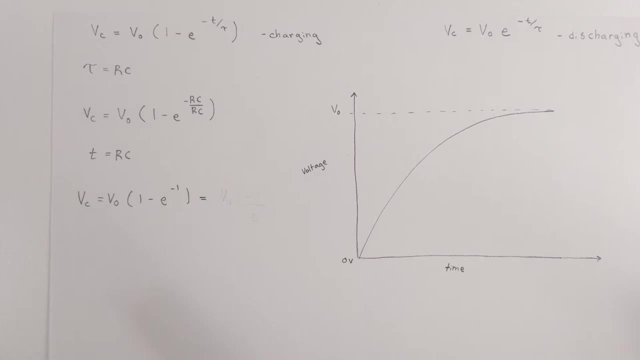 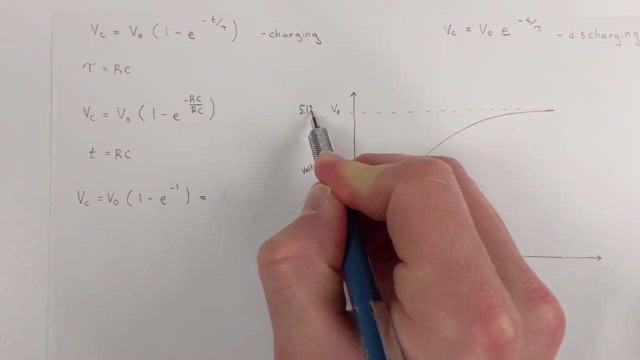 through these variables. V sub C is the voltage of the capacitor, depending on where it is at time. So it is the voltage of the capacitor. V sub zero is the max voltage. The voltage that I'm getting from my function generator is 5.12 load. 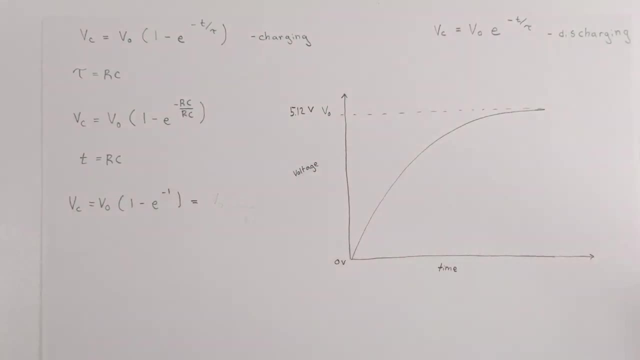 volts. so that's that voltage. now this is 1 minus e to the negative T over tau. tau is the same thing as R times C or resistance times capacitance. so what we're going to do is we're going to set tau equal to RC, and what we end up? 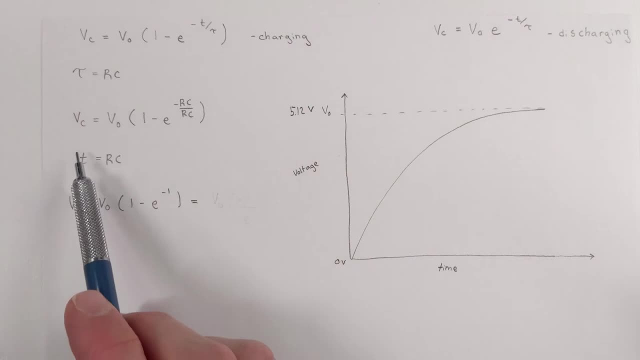 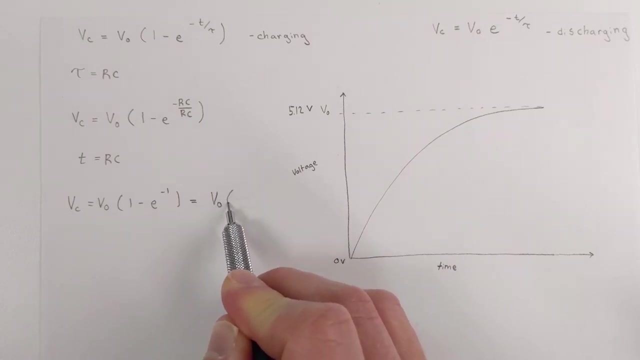 getting sorry. what we're gonna be doing is we're gonna be setting T equal to RC, so that we get negative RC over RC, which is just negative 1, and this is also equal to V sub 0 of 1 minus 1 over e. okay, but you can still work with that. 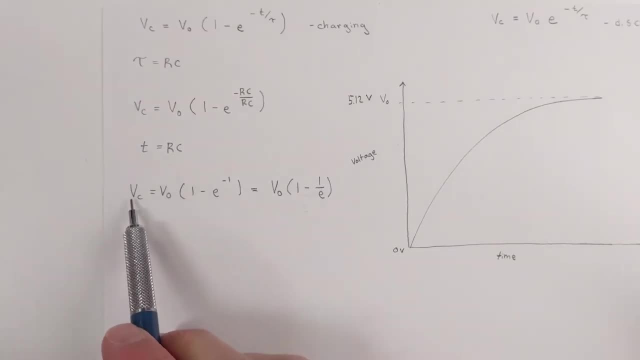 and so we want to figure out the voltage of the capacitor when it is, when it's at this this time. so what we'll get is V sub C is equal to our voltage here, 1, 2 volts times 1 minus e to the negative first. 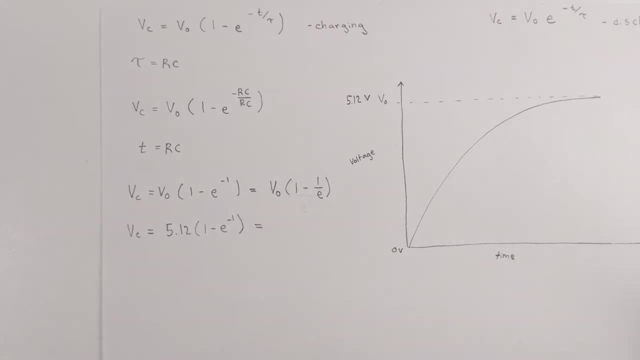 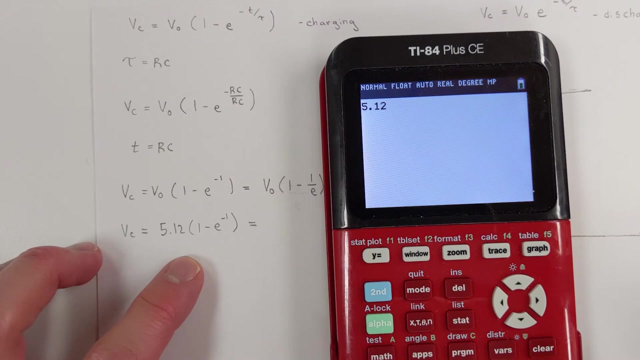 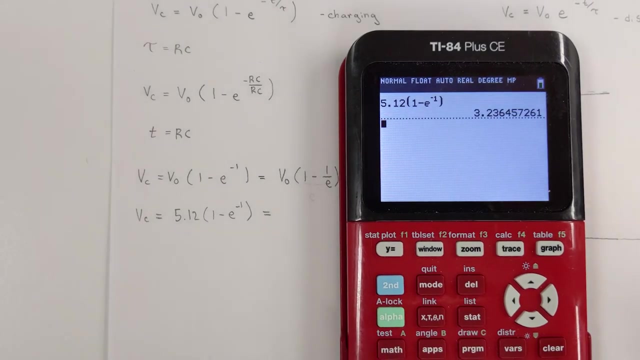 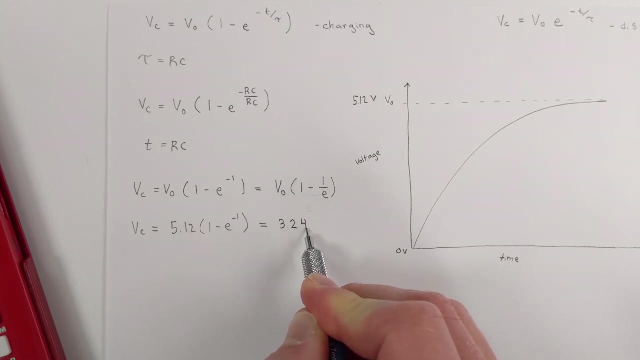 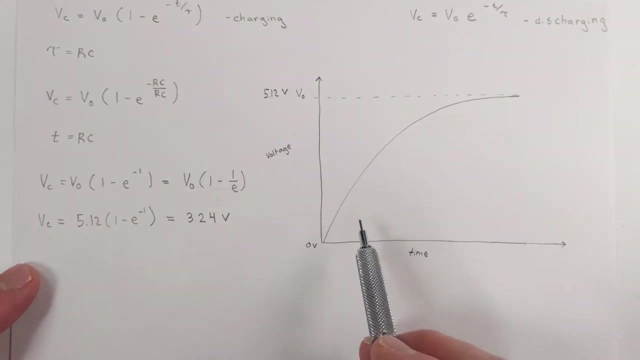 and that's equal to. so that's equal to 3.236, let's just go 3.24 volts. so now we know this voltage we're going to come over to here and we want to find, using our oscilloscope, where, how much time it takes the capacitor to charge up to 3.24 volts. 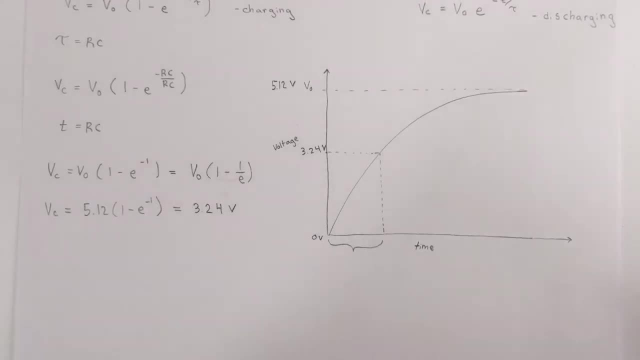 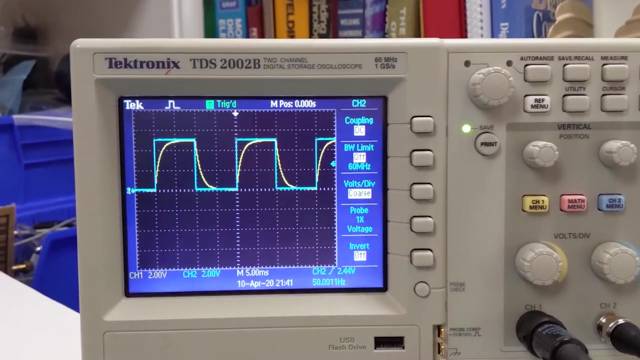 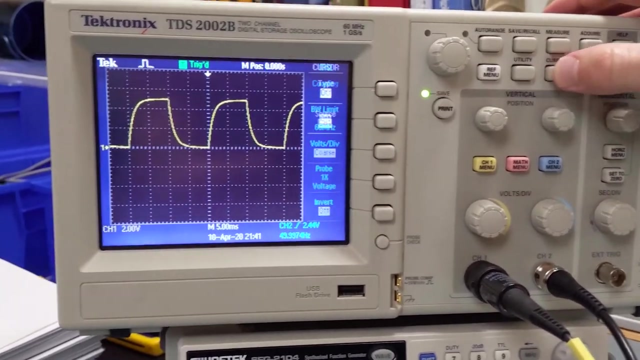 and we want to find this time, so let me show you how you do that. Okay, so how we're going to find. this is we're going to use now. I have a digital oscilloscope, so I've got some cool tools I can use. I can pull up a cursor and I'm going use my牛 if this doesn't work off. 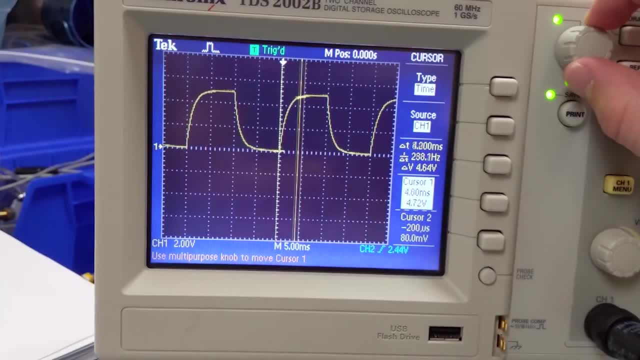 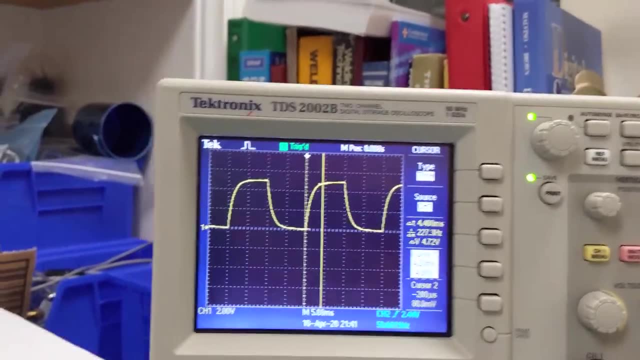 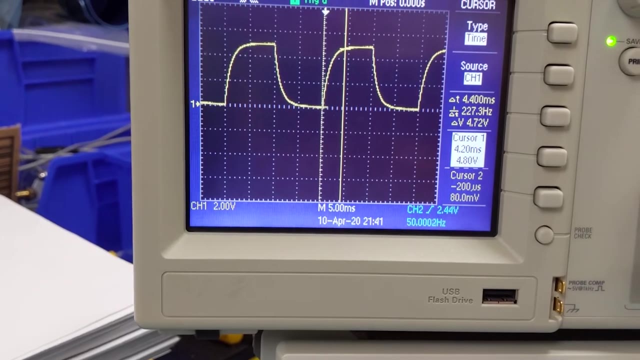 And I can actually select where I want the cursor to be. Now, if you don't have the cursor function, or if you're using an analog oscilloscope, you're just going to have to work with the divisions, making sure to know how much time. 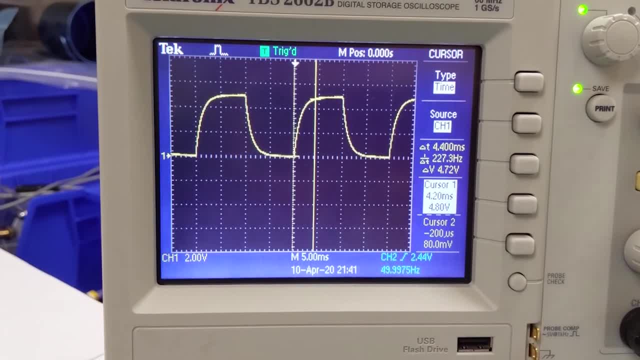 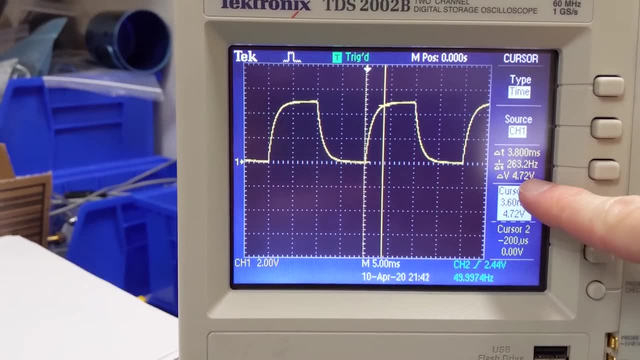 per division. you've got your oscilloscope set at so that you get the proper number, But since I've got this function, I'm going to use it, And so what I've got here is: you can see the voltage here, and I want that to be at. 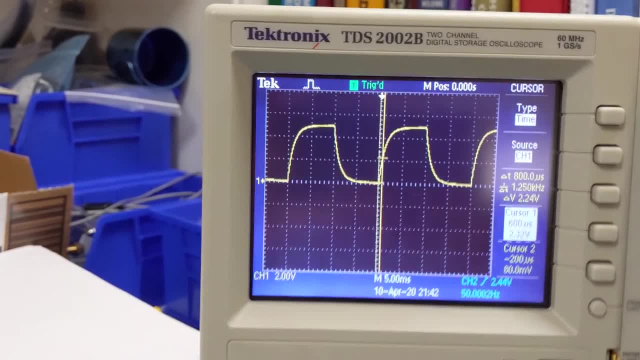 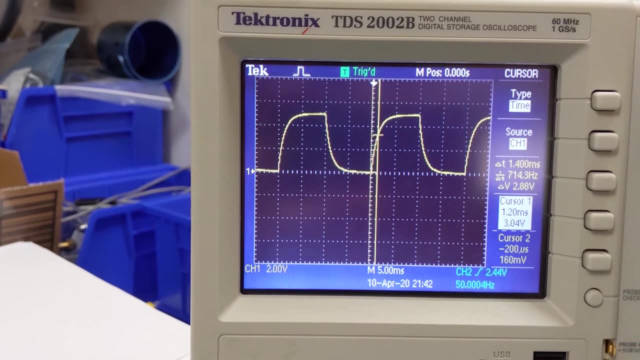 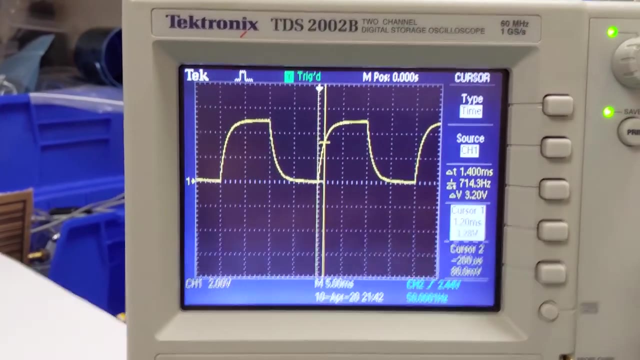 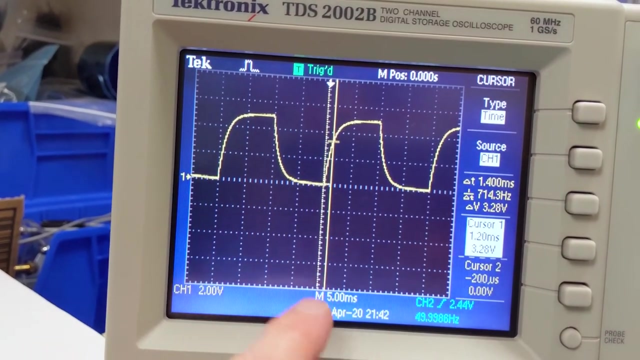 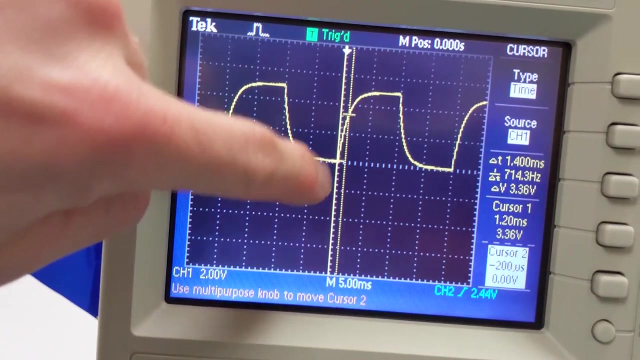 3.24 volts, So it's kind of hard to get there, but okay, 3.2 volts. Now, what that's doing is it is It's taking, It's measuring from this other cursor, which is right here. 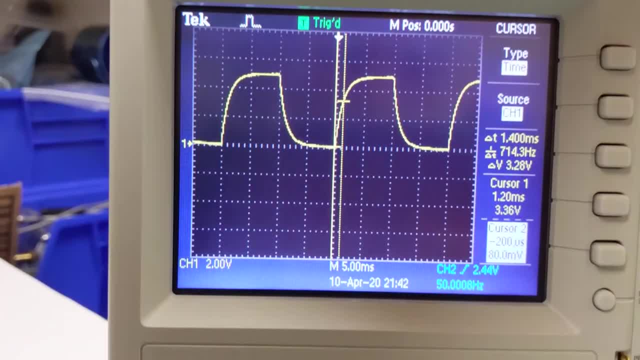 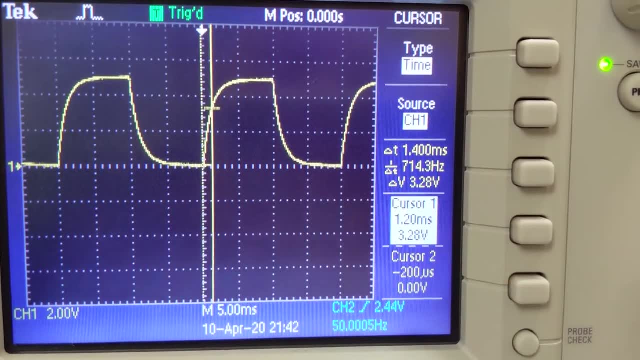 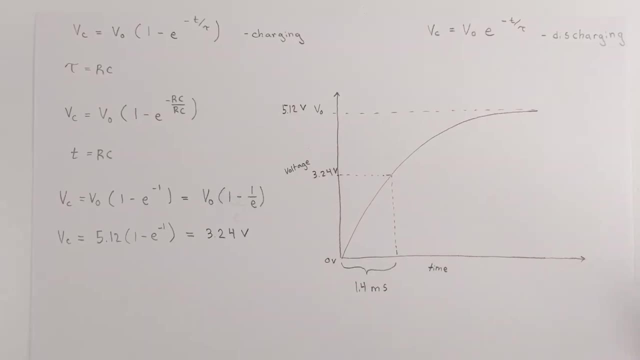 It's measuring that tiny space in between there, And so what I can look at is over here you can see that that delta T is 1.4 milliseconds, So we're going to use that in our equation, All right, So it takes the capacitor 1.4 milliseconds. 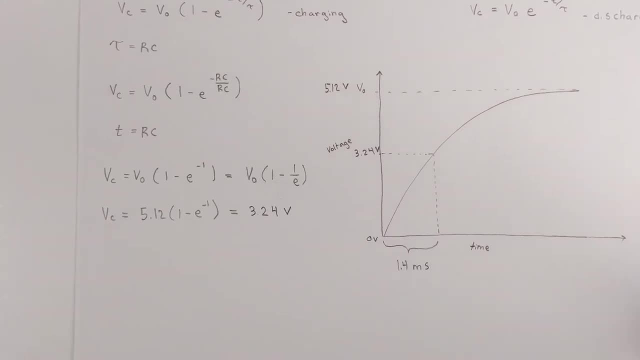 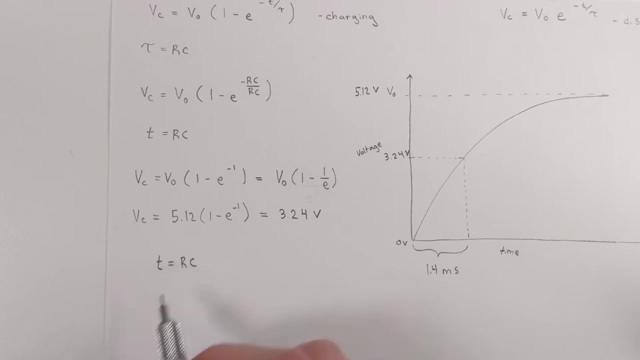 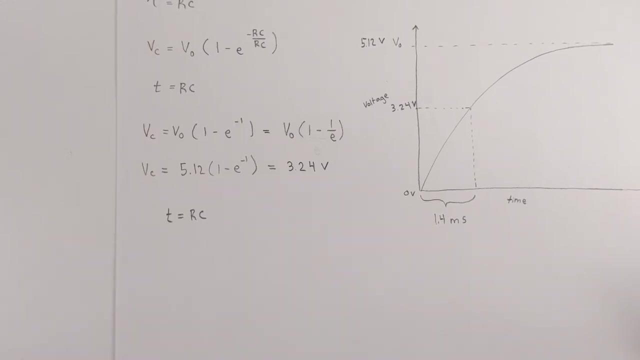 It's going to charge to 3.24 volts, And so now what we can do is: since we set T equal to RC, we can figure out the capacitance. So how we do this is: we're going to rearrange this so we get C on one side. 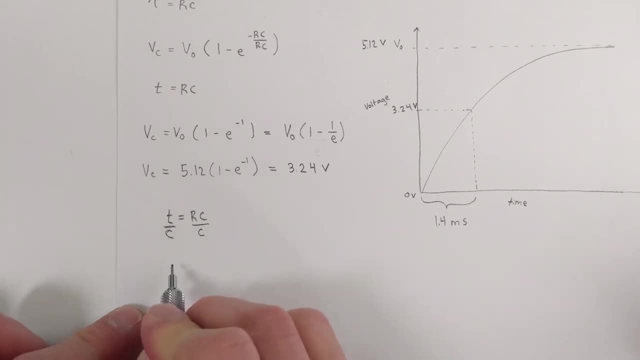 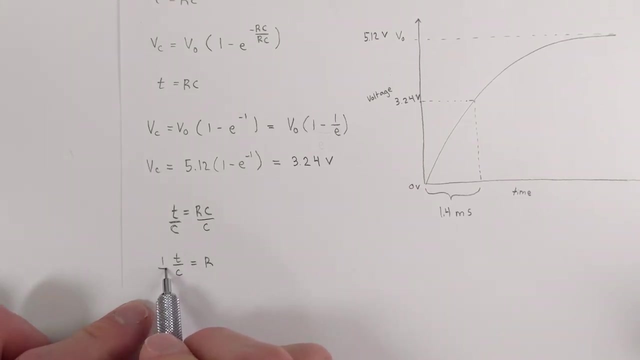 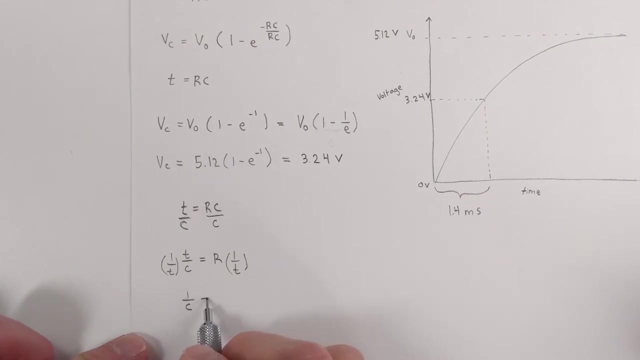 So we divide by C, We get T over C is equal to R. Now we Okay, So Okay, We multiply by the reciprocal, we get T, sorry, not T. we get 1 over C is equal to R over T. Now we take the reciprocal: C is equal to T of R. There's many different ways you. 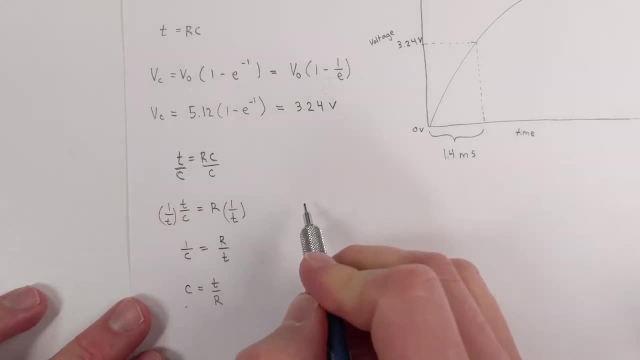 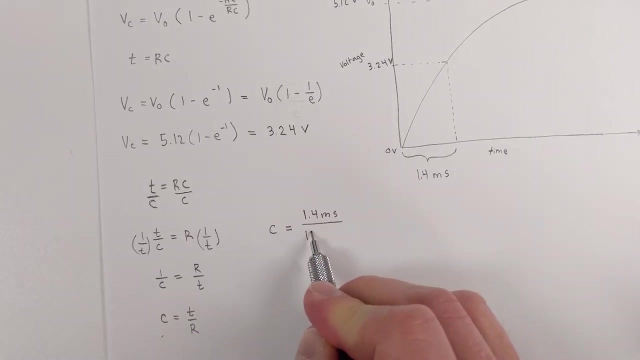 can do that, but that's how I did it, And so C is equal to our time, 1.4 milliseconds divided by our resistance. Now, if you remember back, our resistance was 10,000 ohms, so I'm just going to do 10,000. 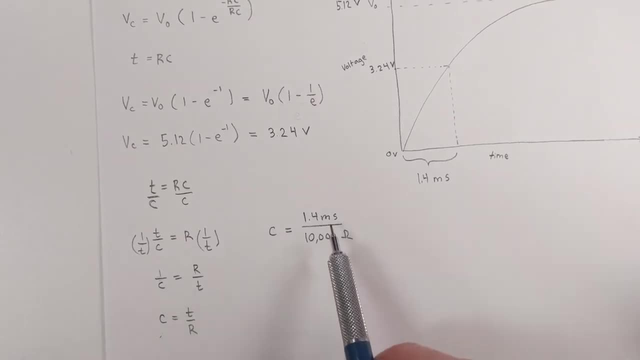 ohms. Now you've got to make sure here that you have this in seconds and then this is in ohms. So I've got to rearrange this. I've got to do 1.4 times 10 to the negative 3.. 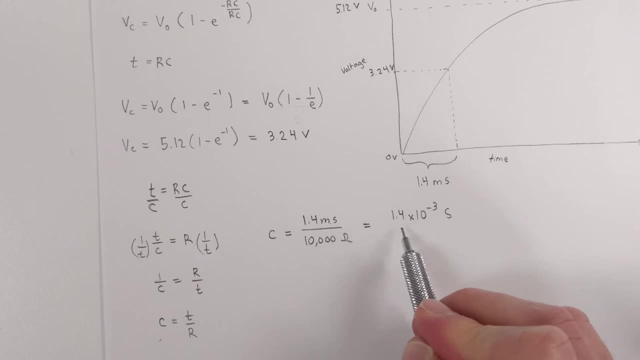 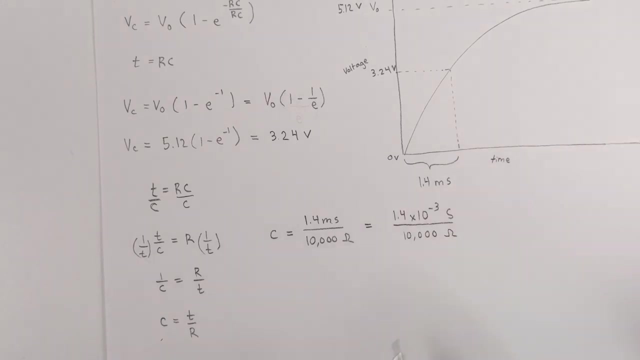 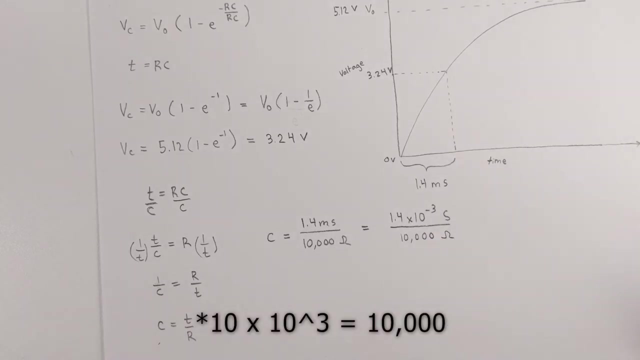 Milliseconds is to the negative 3rd power and then just 10,000 ohms. Now you can also put this into this form. I think it would be 10 to the negative 2, something like that. Don't quote me on that, but we're going to use it that way. 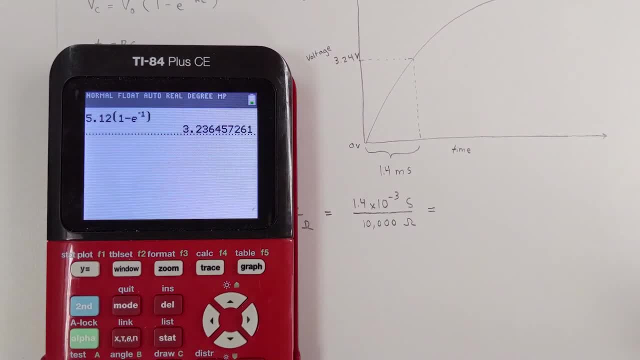 So what we get here? 1.4, I'm going to use E- to the negative 3rd power, 1.4.. 1.4 times 10 to the negative 3 divided by 10,000,. 1.4 times 10 to the negative 7 farads.